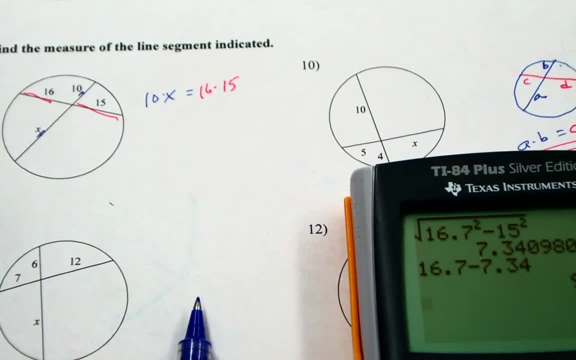 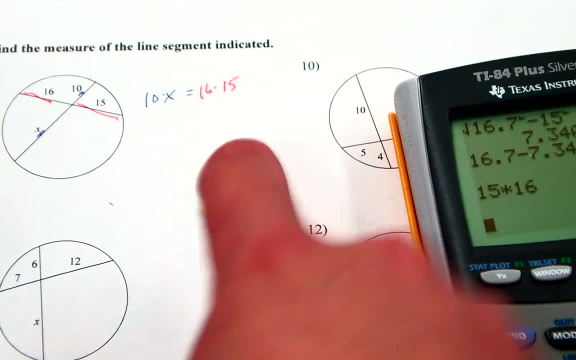 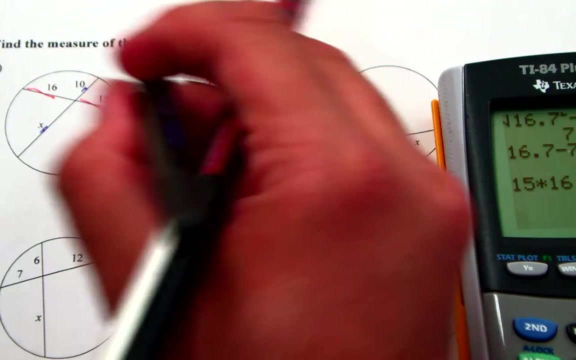 because that would be this and this. So 16 times 15 is 240.. So 10X equals 240, and hopefully you can see from there that just plain old X would equal 10.. And this is a blue length divided by 10.. 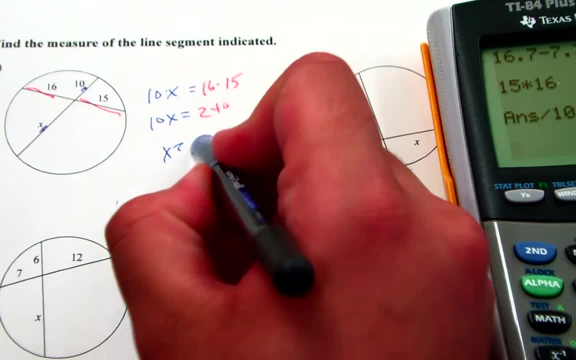 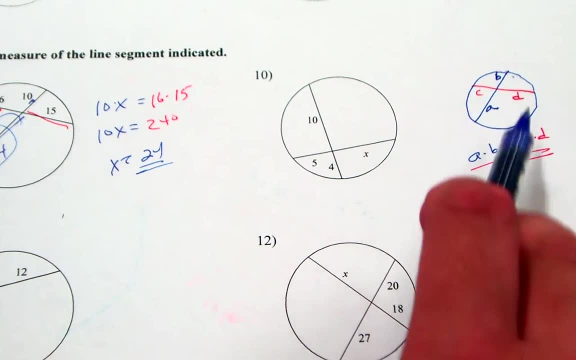 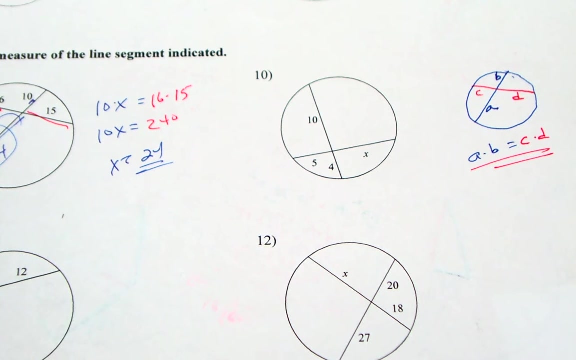 Plain old X would just equal 24.. And it's really as easy as that. It basically boils down to: do you understand, and can you apply this concept, that intersecting chords cut each other in this proportional manner with similar triangles? Looking at number 11 here below, once again very much the same idea. 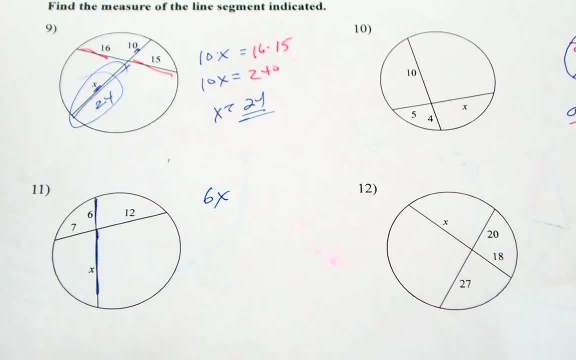 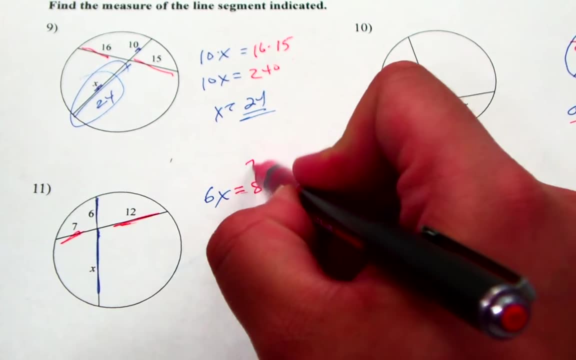 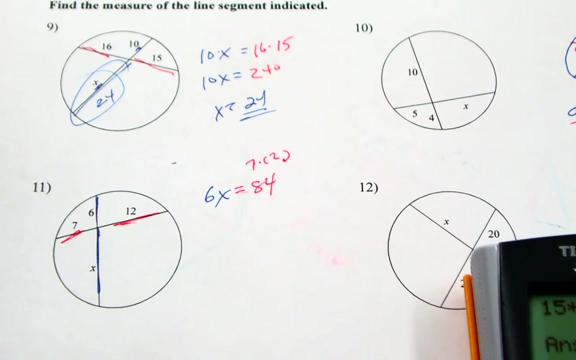 This and this will give us 6X 7 times 12, I believe is 84, so that's this times this, 7 times 12.. So we divide both sides by 6,, 84 by 6, and we get 14.. 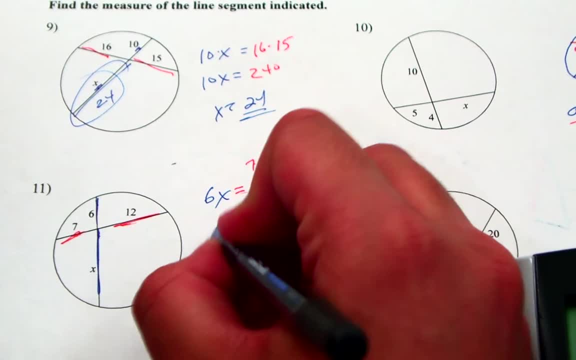 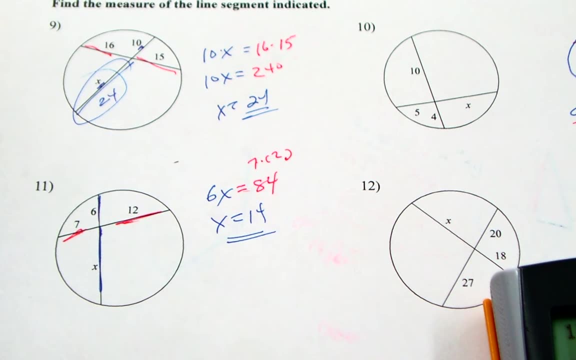 So X is equal to 14.. Now the last example I'm going to show you is a little more complicated. We've got to find the length of segment SQ, and we've got to do so using a little bit more algebra. So we're going to do two things. 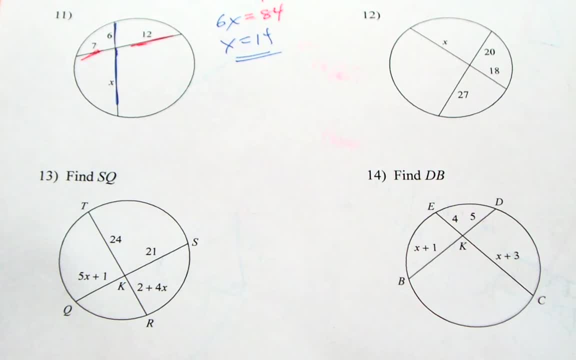 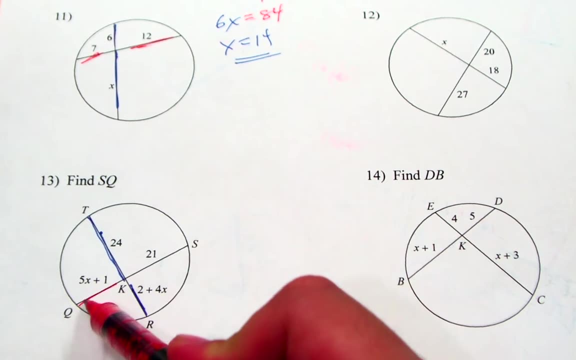 We're going to do two of these. actually, Number 13 says: find SQ. Well, once again, the same principle holds true. 24 times, this is going to equal the same amount as 5X plus 1 times 21.. 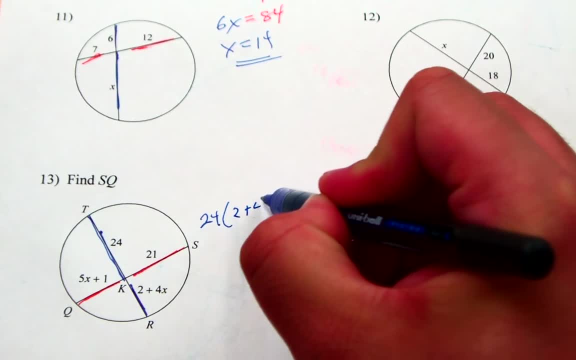 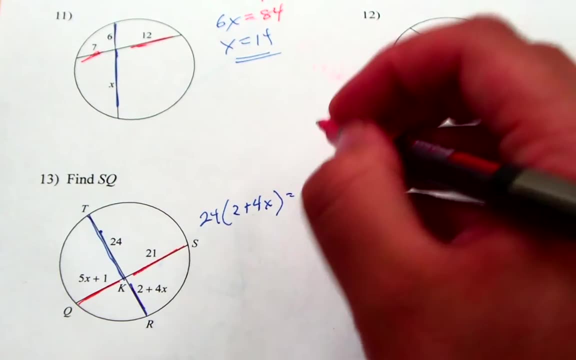 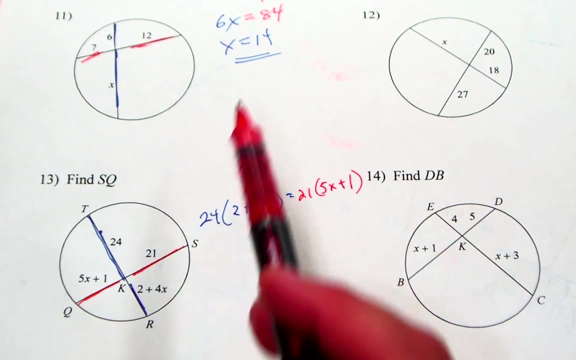 So 24 times 2 plus 4 plus X- sorry, 2 plus 4X, excuse me- is equal to 21 times 5X plus 1.. So this is simply applying the same concept here in a little more algebraic a context. 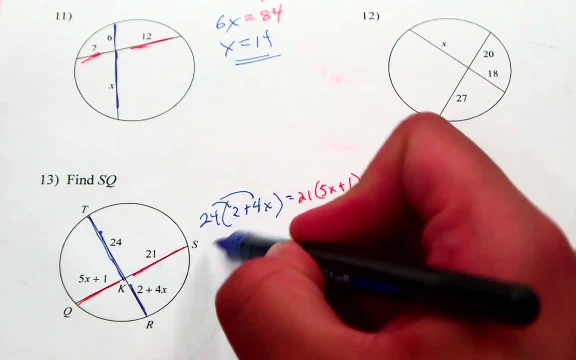 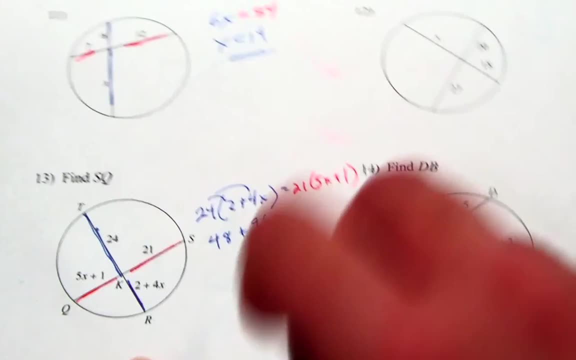 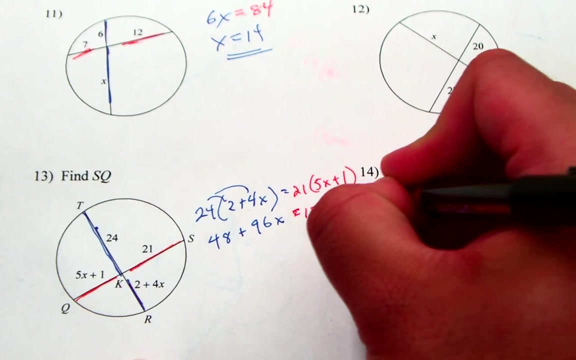 Well, you may remember that to simplify this we need to use a distributive property. So that would be: 48 plus 96X is equal to 105X plus 21,. once again distributing, Gathering my terms all on one side, I'm going to move this 96X across.